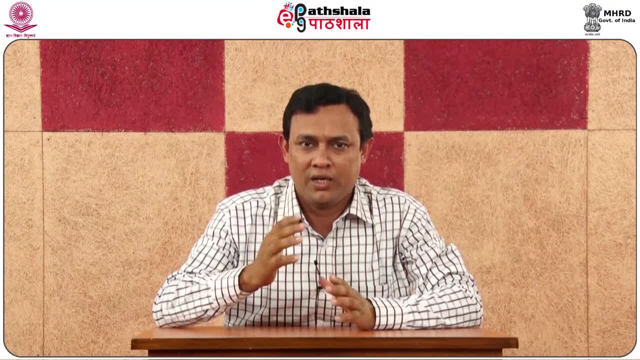 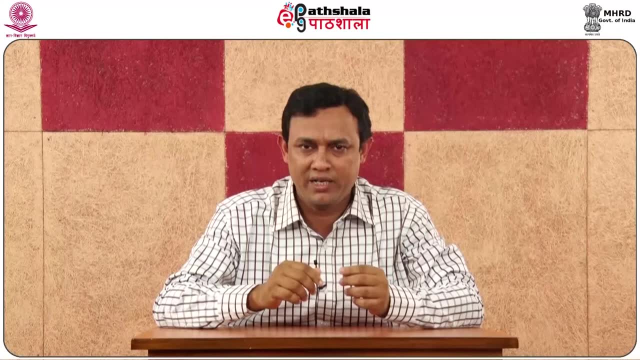 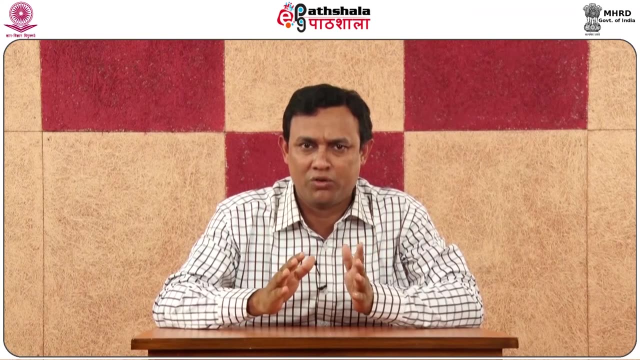 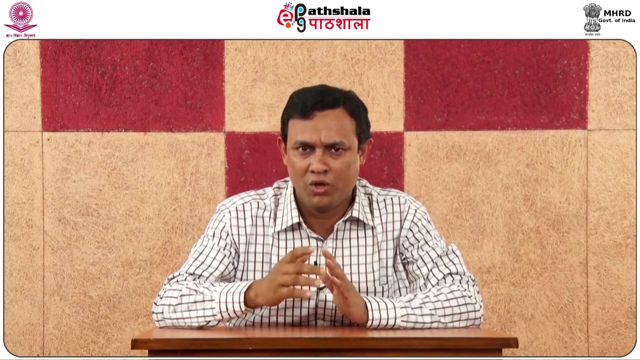 or qualitative geometry. Or for example, let M and N be two letter in English alphabet, Then N can be stretched to N or N can be stretched to M. So M and N are equivalent to a topologist. But if we consider M and the letter B, it is not possible to convert M just by stretching or 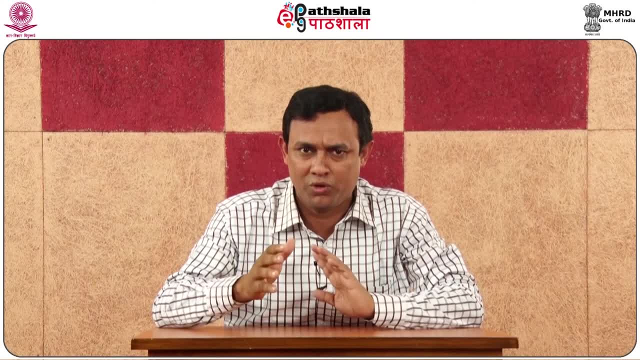 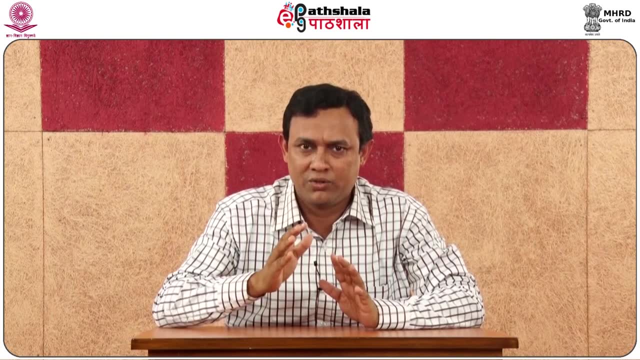 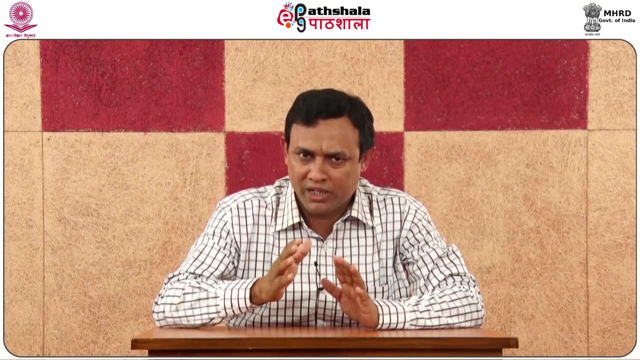 such way to B, So these two will not be topologically equivalent. So these are intuitively saying what we are told. up to that, these are intuitive, So we need some formal definition to to mathematize this. So let us come in the presentation. 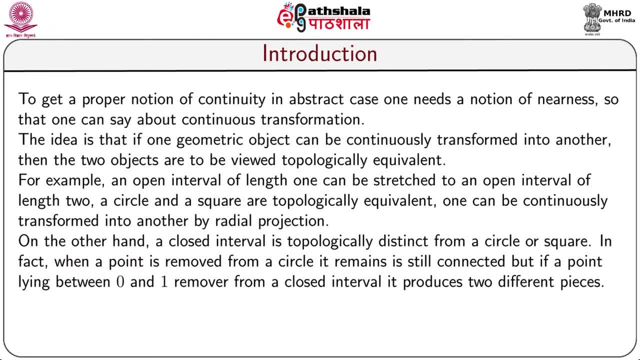 In order to get the notion of continuity in abstract case, one needs a notion of proper definition. So let us move to the notion of continuity in abstract case, That is a particular word that we have already defined: nearness, So that one can say about transformations of geometric 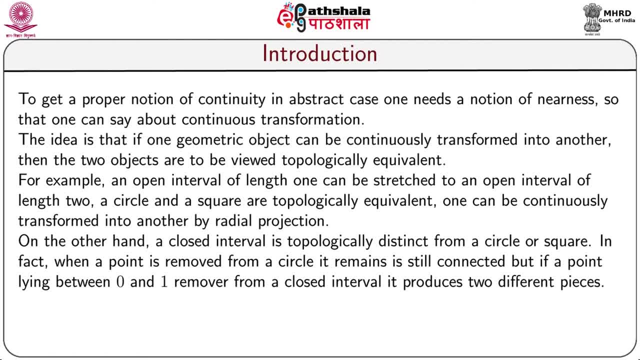 object which preserve nearness. The idea is that if one geometric object can be continuously transformed to another, then they will be equivalent, For example. so let us consider circle. If we observe that closely, that circle can be continuously transformed to a square or a triangle. 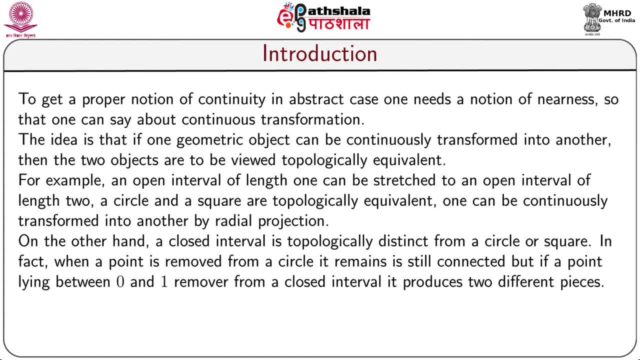 So they are topologically equivalent. or let us consider an open interval of size 1.. Then this open interval can be continuously transformed to another open interval of size 2.. So these two open interval are topologically equivalent. But if we consider an open interval and a circle, these two will not be topologically equivalent. 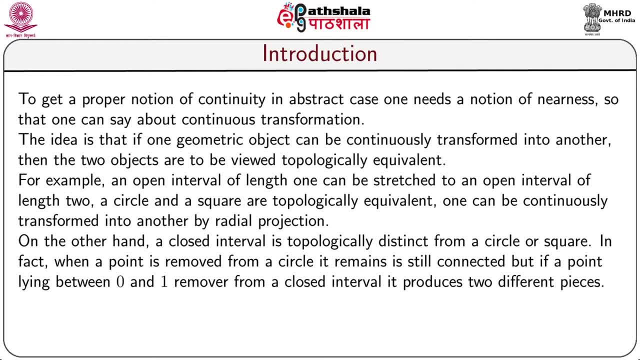 Why? Because this is just intuitively saying that if we take a point from the open interval and if we take a point in the circle, the open interval lefts two components, But the circle lefts just only one component. So this is the problem. 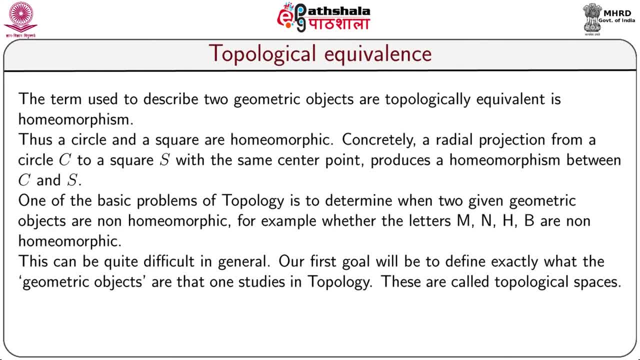 So this is the problem. So the term used to describe two geometric objects that are topologically equivalent is homeomorphic. That means, from now, if two geometric objects are equivalent, we will say that they are homeomorphic. In this terminology, a circle is homeomorphic to a square. 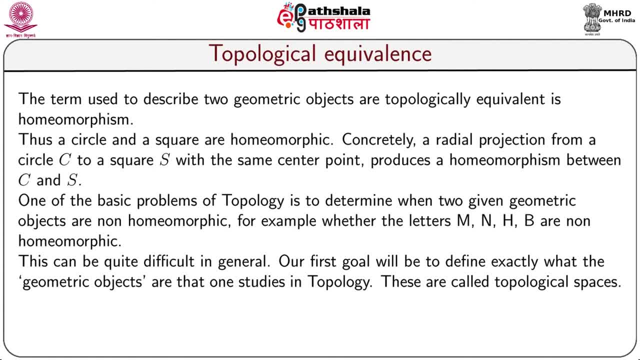 This happens by the radial projection. An open interval of length 1 will be homeomorphic To a greater open interval or smaller open interval. Of course M and N will be homeomorphic, But M and H will not be homeomorphic. This can be quite difficult in general, that whether two topological spaces are equivalent or not, 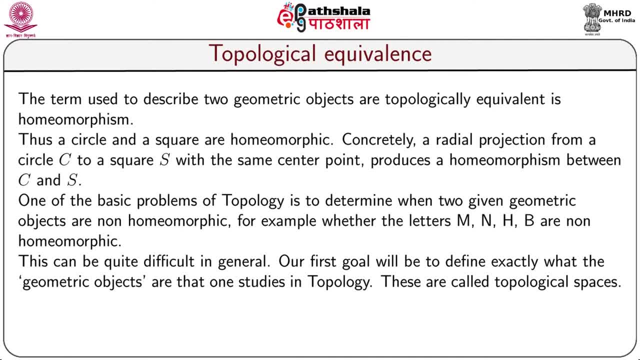 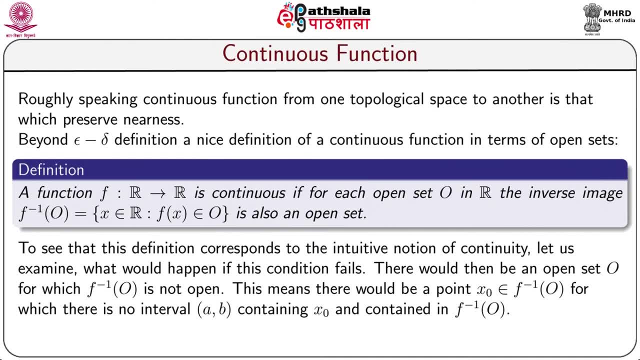 So to show that two topological spaces are not equivalent, it requires a topological space. It requires harder work. But to get the proper notion of topological spaces first we have to get a proper notion of continuity. So let us start from the elementary real analysis. 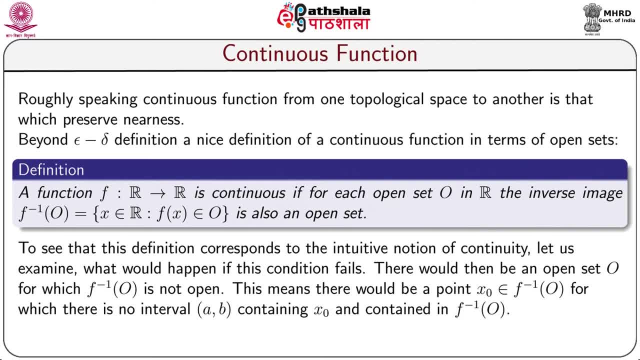 We know that in the elementary real analysis epsilon delta definition of continuity. But this definition also comes in the elementary real analysis. That is, this function: f from R to R is continuous if for each open set O in R the inverse image f, inverse O is also an open set. 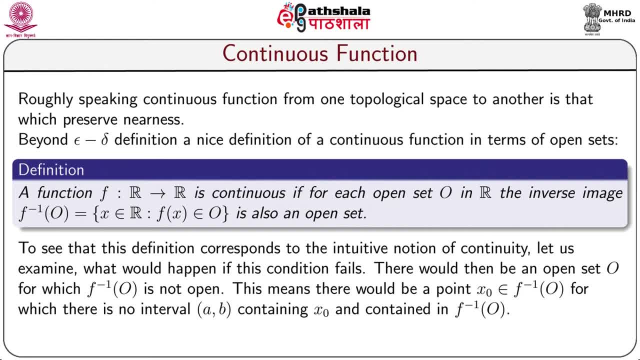 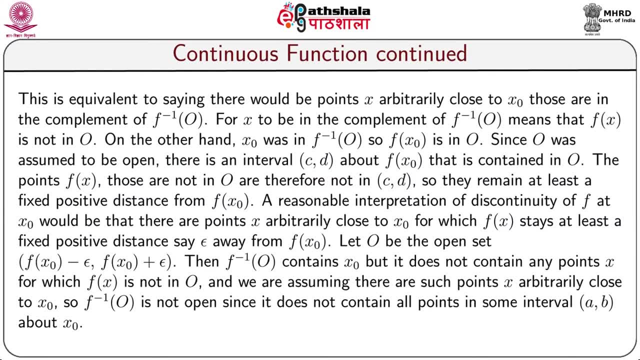 We will use this definition to define continuous function between two topological spaces. This definition in fact preserves continuity. So in trying to find a sentence, in the end if a function, f minus the inverse function of R is continuous, we will need arpeggios. 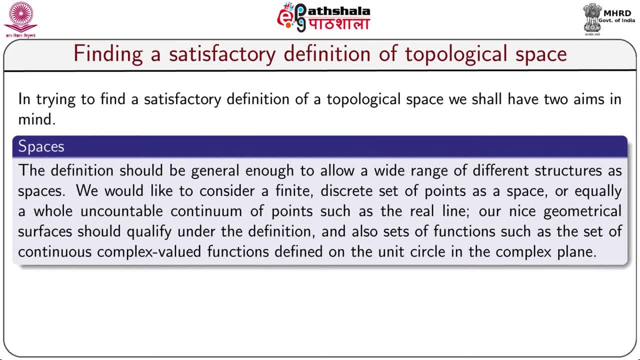 In a satisfactory definition of continuous function or topological space. we would like to consider finite set, discrete set of points as a space or equally whole, uncountable continuum of points, such as rail line, one of our nice geometrical surface, should qualify under this. 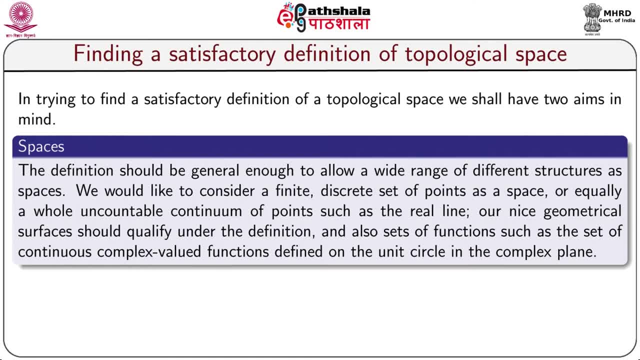 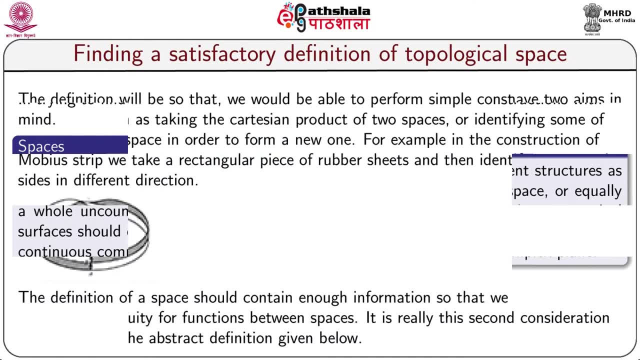 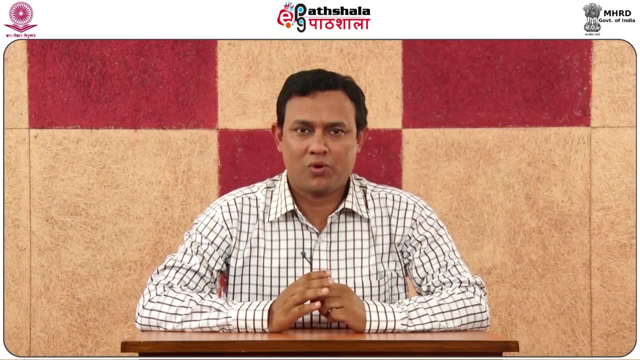 definition And also sets of functions, such as the set of continuous, complex, valued functions defined on the unit circle, on the complex plane. Let us consider an example, a very beautiful example of topological spaces, which is called Möbius strip. One beautiful example of geometric object is Möbius strip, which you have seen in the 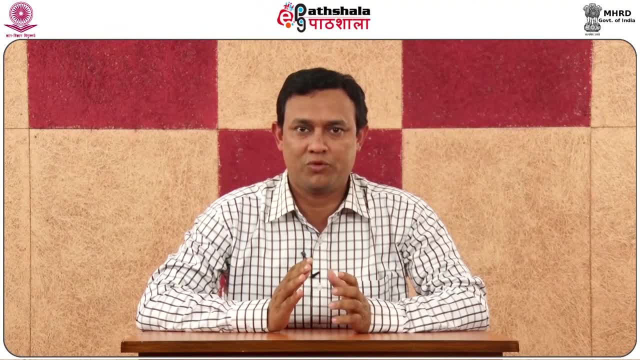 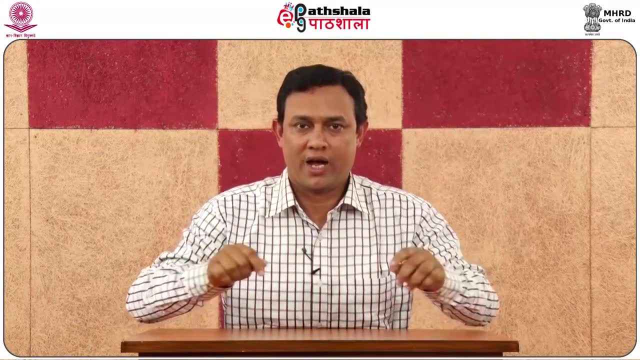 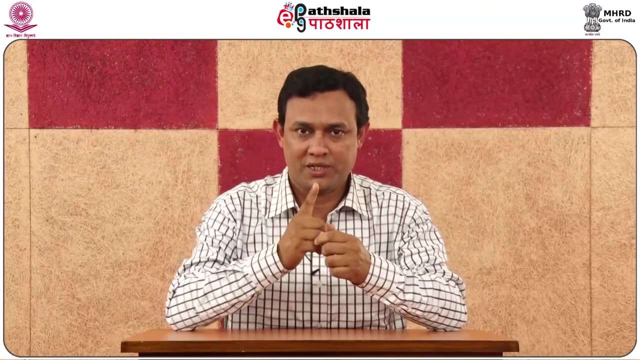 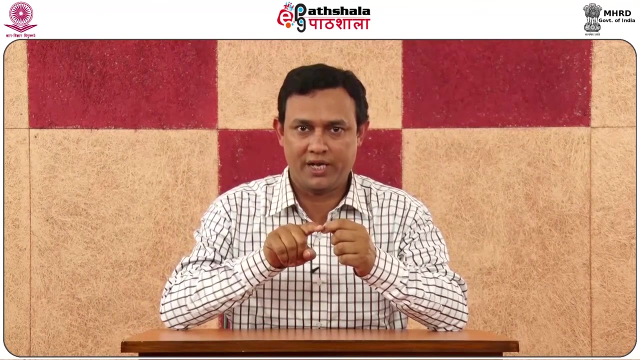 last slide What we do to construct a Möbius strip. Let us take a plane piece, A piece of rectangular paper, then identify the left side and right side, making the direction opposite. Then what happens? If one starts to run from a point, then when he returns back to that point, again his direction 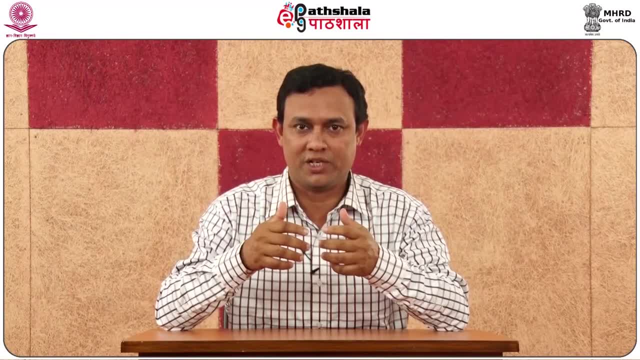 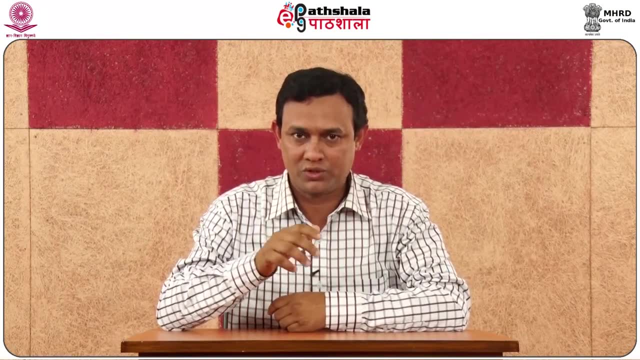 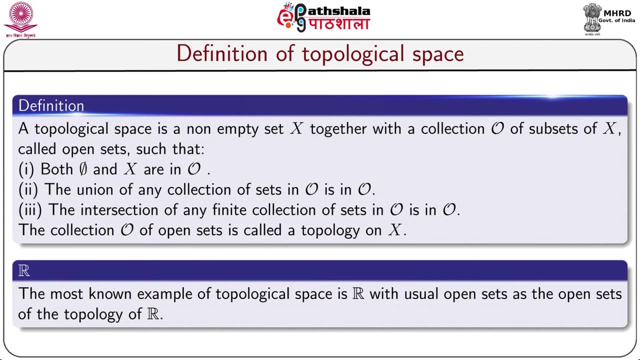 changed. So this is orientation. preserving This Möbius strip will be act as a very important example in our whole study. Now we will give a formal definition of topological space. By a topological space we mean a non-empty set- X- and a subset of power set of X, which 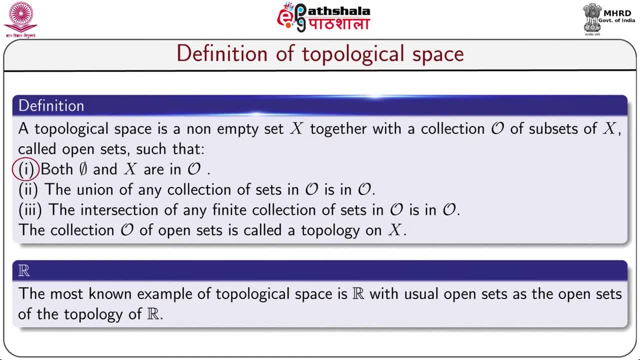 satisfy the following properties. First one is both empty set and whole set. X is in R in O. Second one is O is cosine right closed under arbitrary union. third one is O is closed under finite intersection. Then O will be called a topology on X and X and O simultaneously will be called a topological. 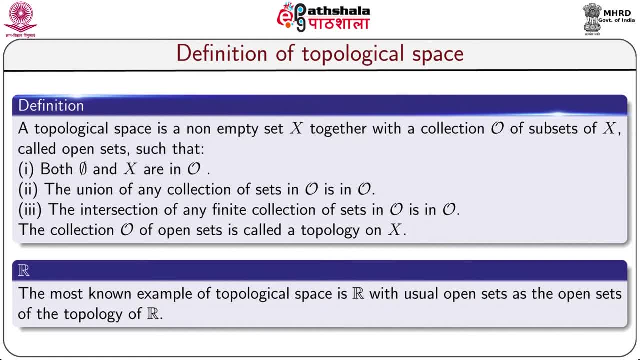 space. From now we will avoid O and generally we called X as a topological space. Our most known example of topological space is a set of real numbers. This is called generally called usual topology Here. what we know, the FD, encouraging our entrepreneurial 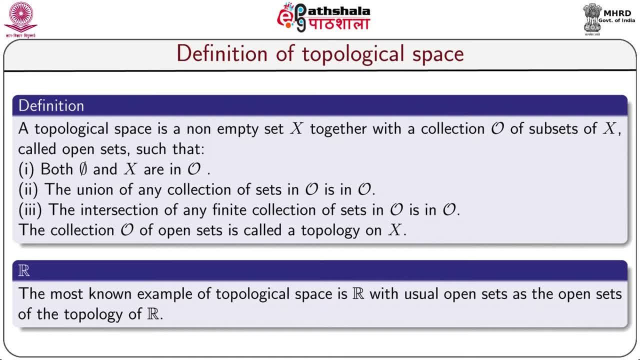 analysis. what are open set Here? open set are also those and we can easily verify that open sets here satisfy these properties. That means in R an empty set is open, the whole R is open. We know in R arbitrary union of open set is open, finite intersection open sets is open. 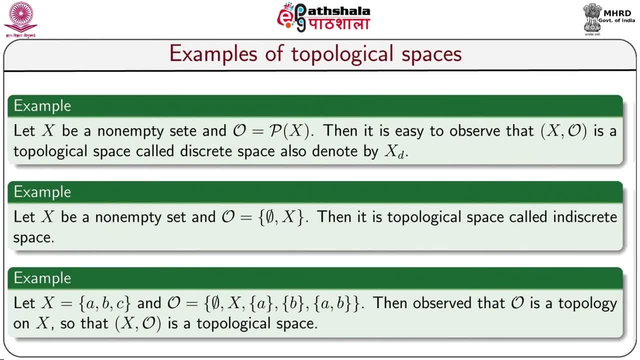 Let us give some other examples. Let X be a non-empty set and script O be the power set of X. Then it is easy to observe that XO is a topological space. it is called discrete topological space. In mathematical situation, discrete topological space is extremely important. 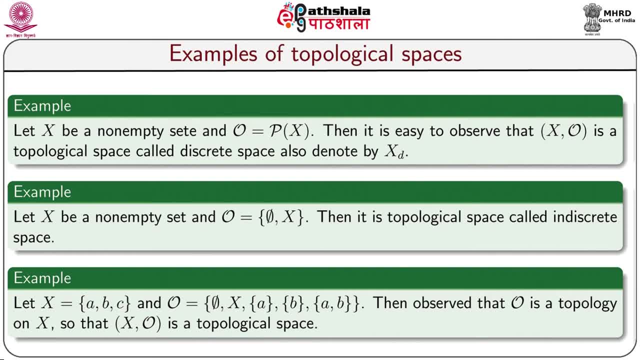 Another example of topological space is indiscrete topological space. Here we take as open sets only empty set and X. This is not so much important topological space. but I have given just for example. Let us consider another example of topological space. 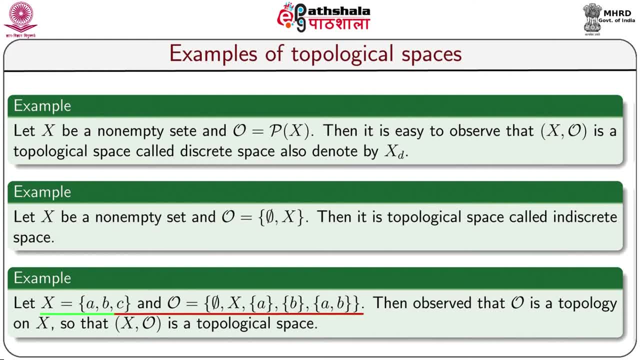 Let X be the finite set, A, A, B, C and script O be considered. Script O contains empty set, whole set X, singleton set A, singleton set B and the set containing A- B. We can verify that this is a topology on X because this is closed under arbitrary union. 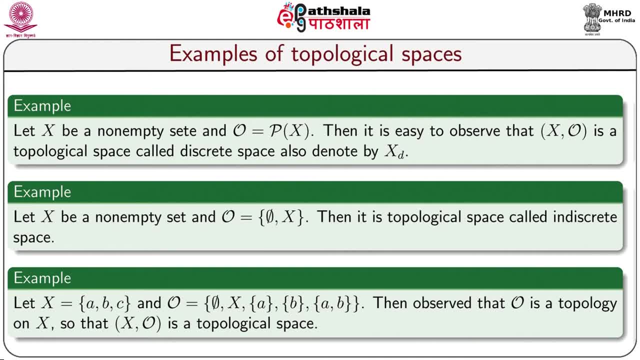 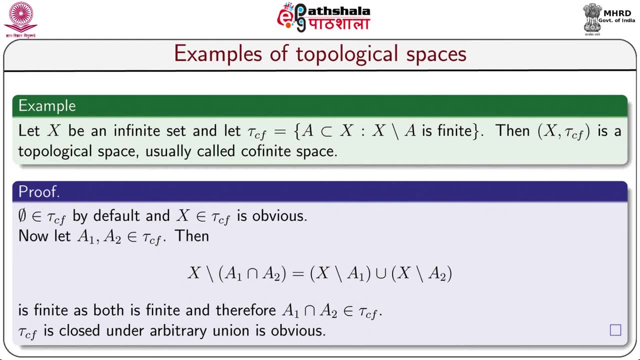 and closed under finite intersection. So this is also a topological space. Let us consider some more examples. Let us consider some more examples. Let us consider some more examples. Here we have a more important topological space. This is called co-finite topological space. 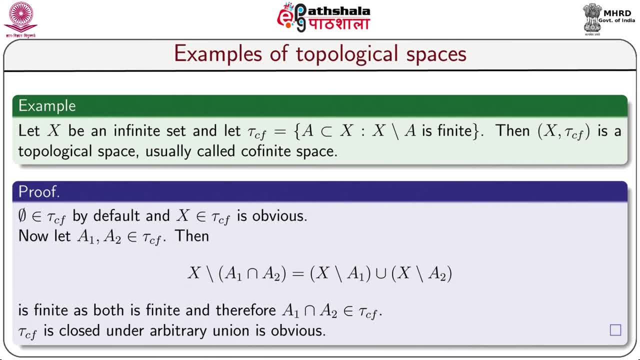 So how this topological space is defined. Let us consider an infinite set, X, and let us consider tau CF is the collection of all those subsets of X whose complement is finite. Then we can prove that tau CF is a topology on X. Then we can prove that tau CF is a topology on X. 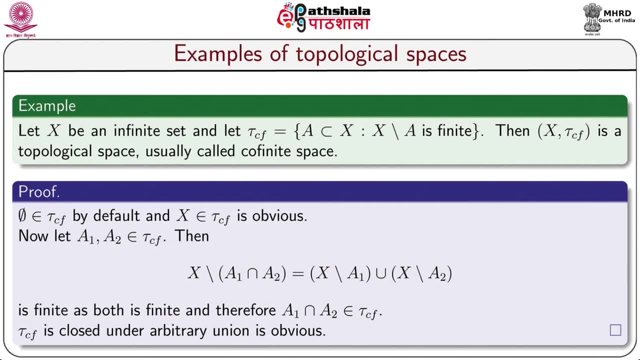 cf is called co-finite topological space. The proof is very easy. You can see the proof: Empty set belongs to tau cf by vacuously: x obviously belongs to tau cf. Now let us consider a1 and a2 belongs to tau cf. That means complement of a1 and a2, finite Then 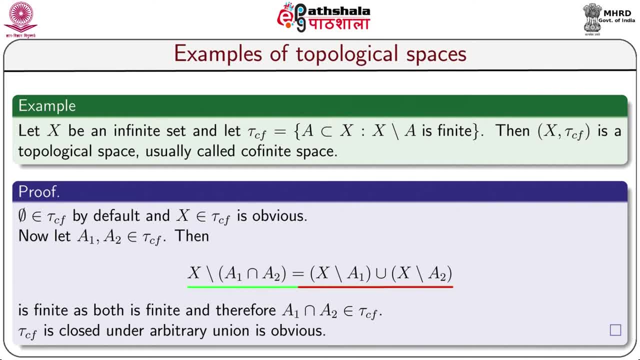 x minus a1, intersection a2 is equal to x minus a1, union x minus a2.. Now, as a1, a2 both belongs to tau cf, then x minus a1 is finite. x minus a2 is finite, So right hand side is finite. 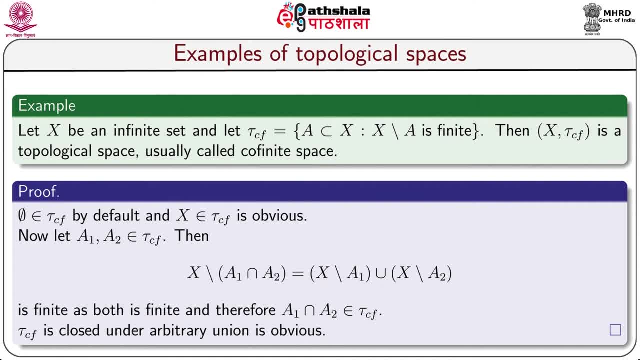 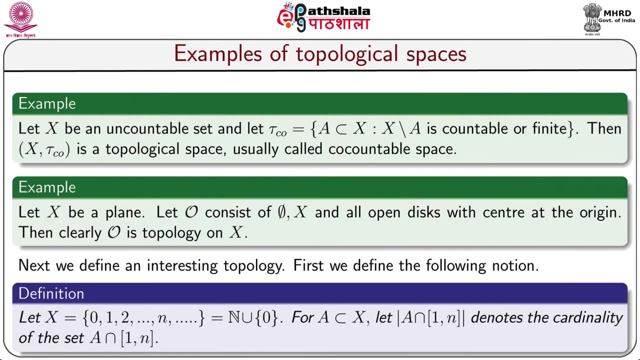 That means x minus a1. intersection a2 is finite. That means a1 intersection a2 belongs to tau cf. So tau cf is closed under Finite intersection And it is obvious that tau cf is closed under arbitrary union. This is a generalization of the previous example. There we told about that co-finite topological. 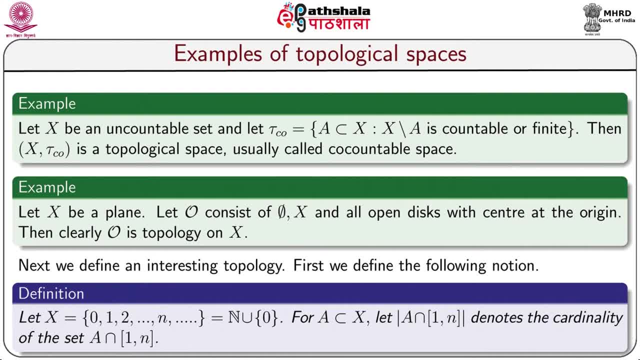 space. Now I am telling about that co-countable topological space For this. so let us take a set with cardinality at least uncountable. So let us take a set with cardinality at least uncountable. So let us take a set with cardinality at least uncountable. 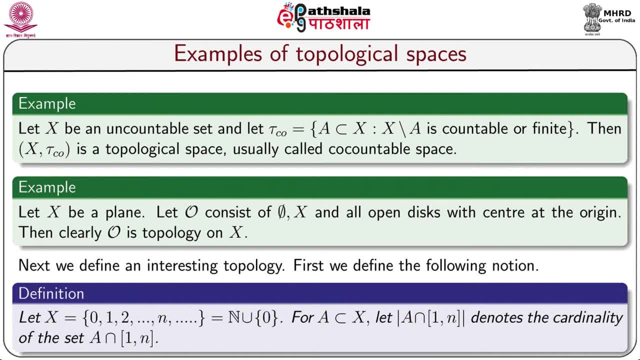 So let x be an uncountable set and consider all those subsets of x whose complement are countable. Then this collection will be a topology on x. Generally this is denoted as tau, co and called co-countable. topological space Proof is almost as the above, So we 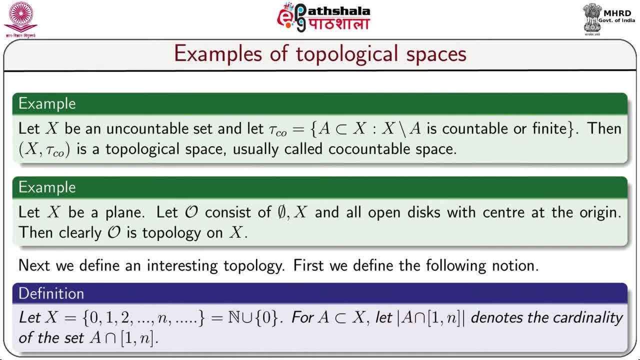 will not repeat the proof here. Another example: Let x be a plane that means R2.. And let O consists of empty set and x And all open digs with center at origin, Then clearly O will be a topology. on x, Next we define: 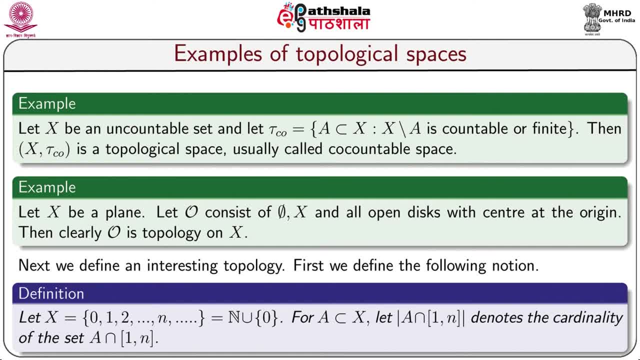 an interesting topology. This consists of some number theoretic flavor. Before that, we define the following notion: Let x be the set of all empty sets, So let x be a plane and x will be called co-countable. And this particular notion is the composition of an all-negative integer. That means 0,. 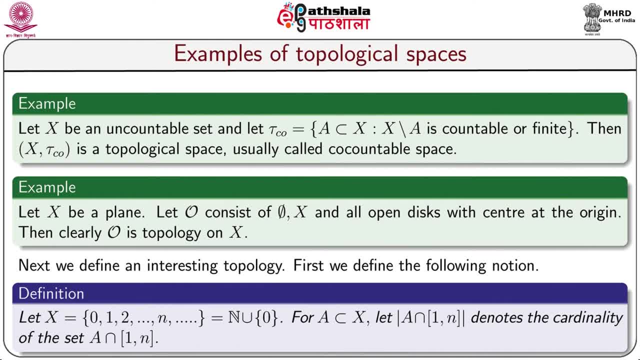 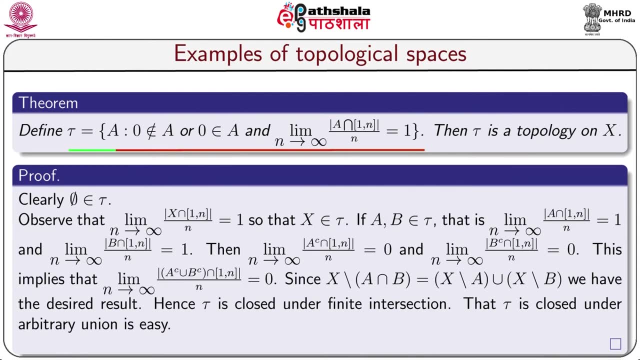 1, 2. And for any subset of x. For a subset of x, let us consider the cardinality of A intersection 1 to N as this. Let us define: tau is equal to all those subsets of x, such that that 0 does not belong to A. 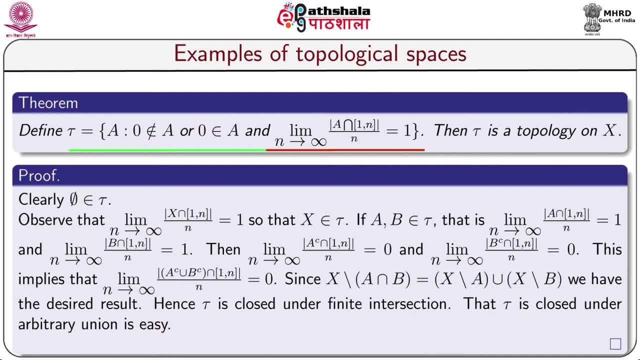 and 0 belongs to children. So this is also co-consp评 The reason we designing division 0 belongs to A and limit n tending to infinity. cardinality of A intersection 1 to n by n is equal to 1.. It can be proved that then tau is a topology. on x, Clearly empty set. 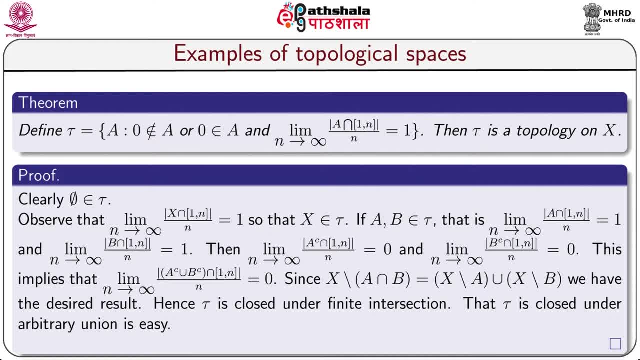 belongs to tau and obviously x belongs to tau because x intersection 1 by n, its cardinality by n. this is equal to 1.. So the limit will go to 1.. Now let A belongs to tau. that is limit of cardinality of A. intersection 1 to n by n is equal to 1 and similarly limit. 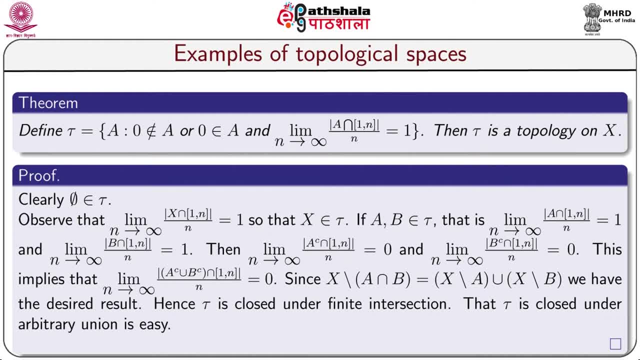 of cardinality B intersection 1 to n is equal to 1.. 1 to n by n is equal to 1.. Then limit cardinality of A complement intersection 1 to n by n is equal to 0 and limit cardinality of B complement intersection 1 to n by n is equal to 0. This: 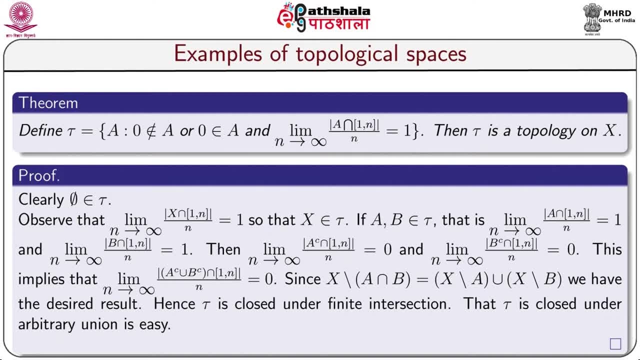 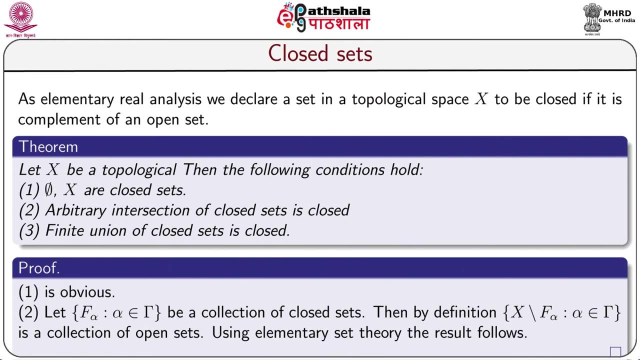 implies that limit cardinality of A complement union B, complement intersection 1 to n by n is equal to 0. Since x minus A intersection B is equal to x minus A union x minus B, we have the desired result As elementary real analysis. we declare here a set in a topological 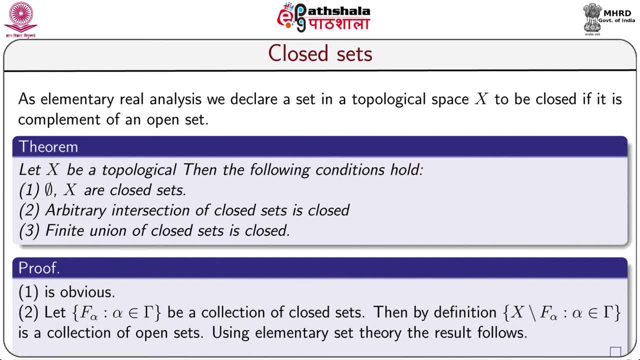 space to be closed if its complement is open. So in a topological space a set will be called closed if its complement is open, Then following can be proved Theorem: Let x be a topological space, Then the following conditions hold: Number 1, empty set and x are closed sets. Number 2, arbitrary intersection. 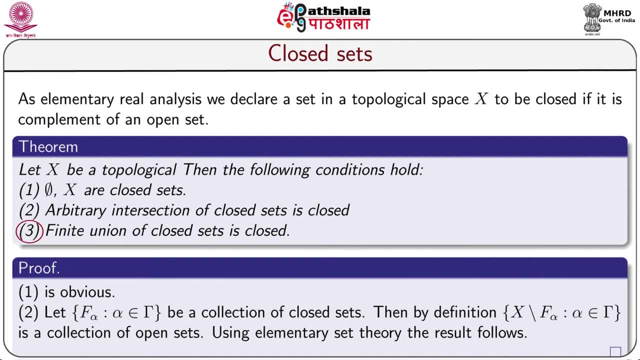 of closed set is closed. Number 3, finite union of closed set is closed. Empty set and whole set x are closed because their complements are open set And rest of 2, finite union of closed set is closed. So let us consider the arbitrary collection of closed sets. Let 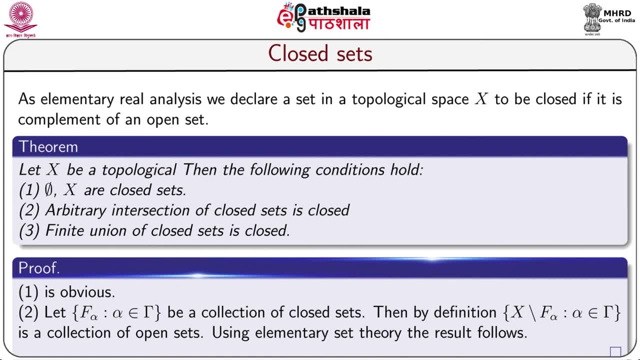 us consider it as f alpha, such that alpha belongs to gamma, where gamma is an index set, Then, by definition of closed sets, each x minus alpha is an open set. So this is a collection x minus alpha, such that alpha belongs to gamma, is a collection of open sets. So 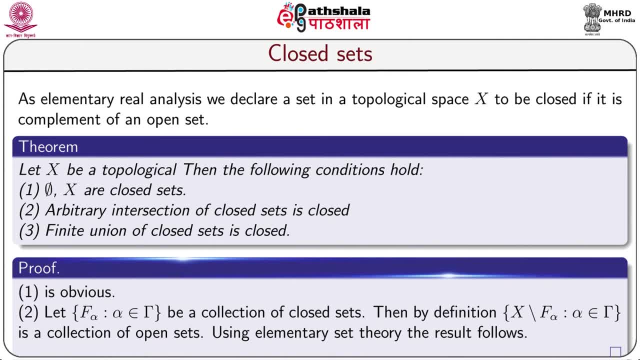 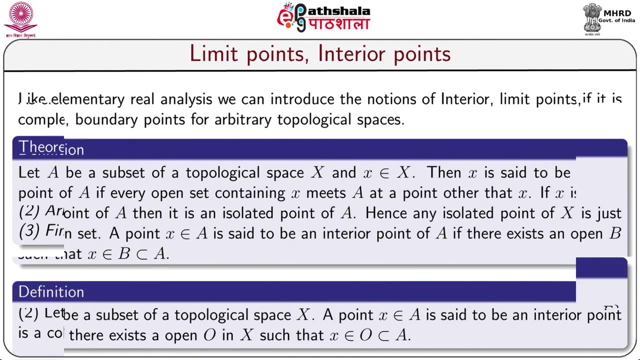 Since open sets are closed under arbitrary union, so their union will be open. That means as their union is open, its complement is closed. That means arbitrary collection of closed set is closed. Again, as elementary real analysis we can define limit points, interior points in arbitrary. 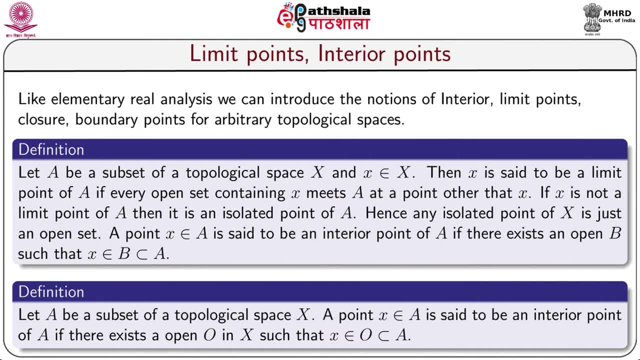 point, topological space also. So let us start the definition. Let X be a topological space, a subset of X, X be an arbitrary point of the topological space, Then X will be called a limit point if any open set containing X intersects A in a point. 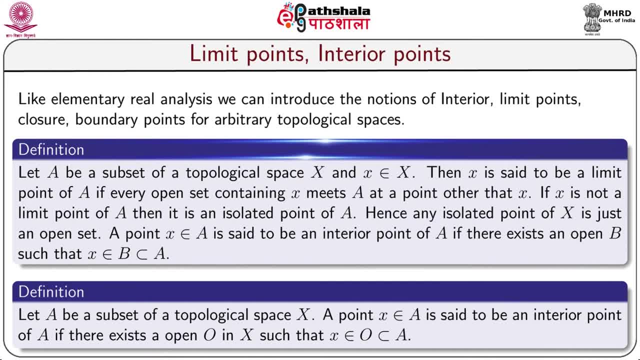 other than X. For example, in the usual topological space R, every real number is a limit point of the set of rational number, or every real number is a limit point of the set of irrational number. In arbitrary topological space, a point which is not a limit point will be called an isolated. 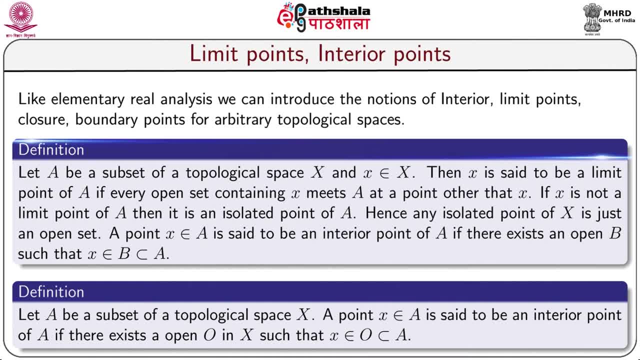 point. Now let us define. Let an appear is called interior point definition. Let A be a subset or a topological space, X and X will be a point in A. then X will be called an interior point of A if there exists an open set. 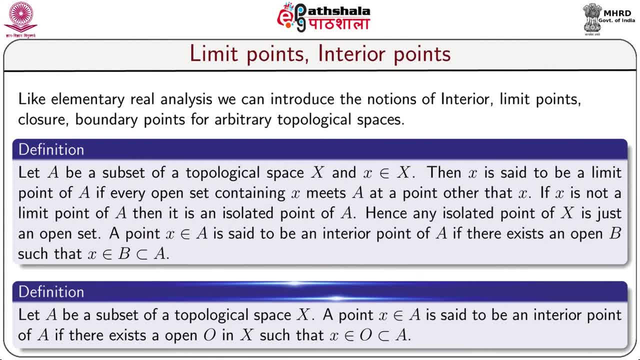 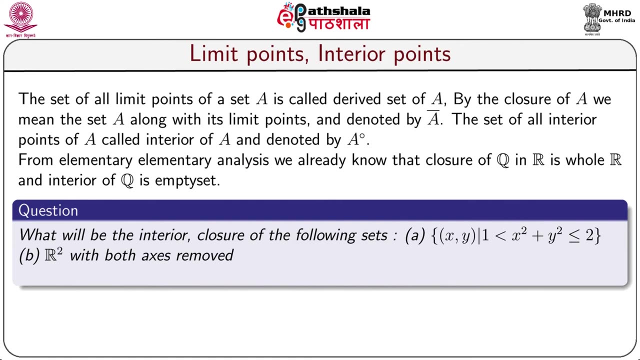 Containing x, which is contained in a We know From elementary real. Unless A set A is open if, and only if, each of its points is an interior point, that will hold here also. The set of all limit points of a set A will be called derived set. 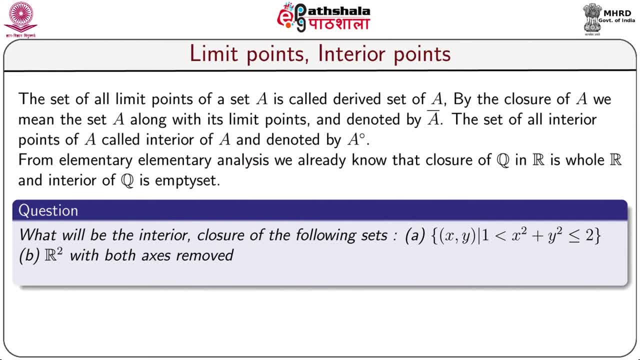 By the closure of A we will mean A along with limit points and it will be denoted by A bar. The set of all interior points of A will be denoted by A interior. So what will be the closure of Q in the usual topology of R? 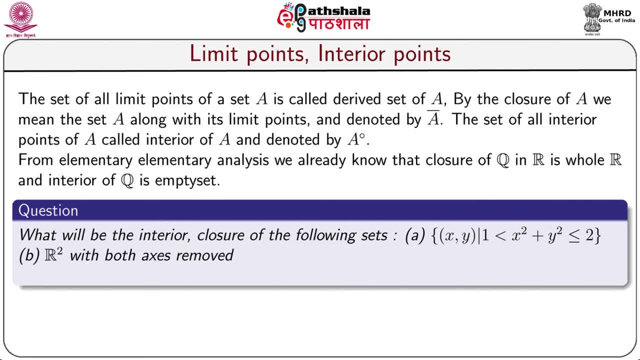 Closure of Q will be whole R and interior of Q will be empty set in the usual topology of R. Let us put a question: What will be the interior and closure of the following sets? First one is all x, y, such that 1 less than x square plus y square less or equal to 2.. 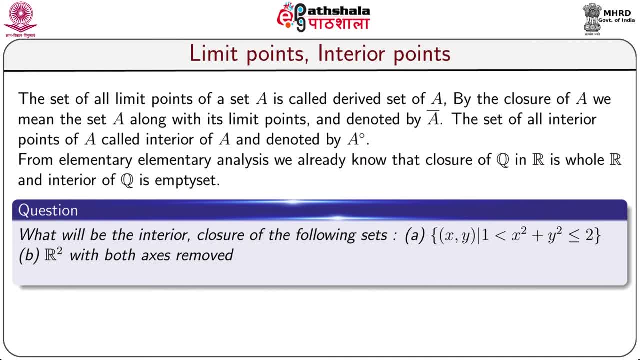 That means it is an annular region. The outside boundary includes, then, this annular region, but the inside boundary is not in the annular region. So what will be the closure In the closure inside boundary will include and to determine the interior, just, we have 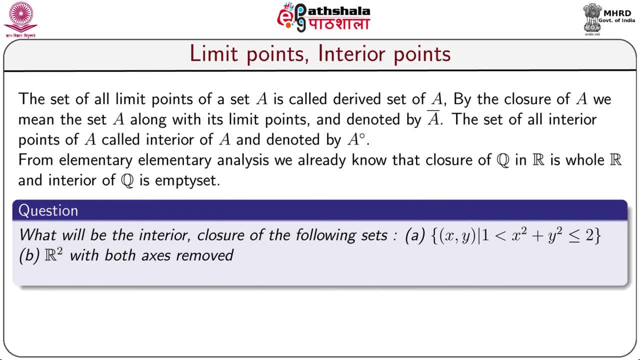 to exclude the outside boundary. Now another question: what will be the closure and interior when both axis have been removed from R2?? When both axis have been removed from R2, its closure will be whole. R2 and interior will be the same. 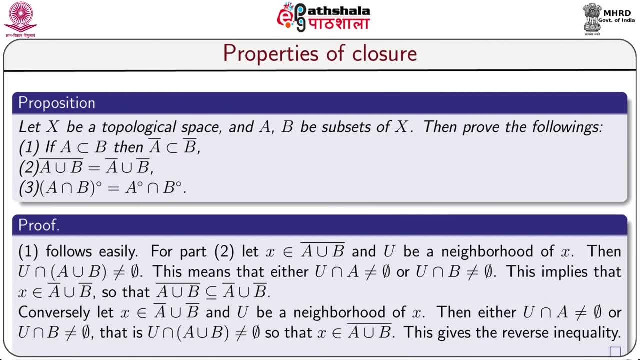 These are the some following properties, some easy properties of closure. Let x be a topological space. A, B, B2, subsets of A, Then let us the following will hold Number one: if A subset of B, then A bar will be contained in B bar. 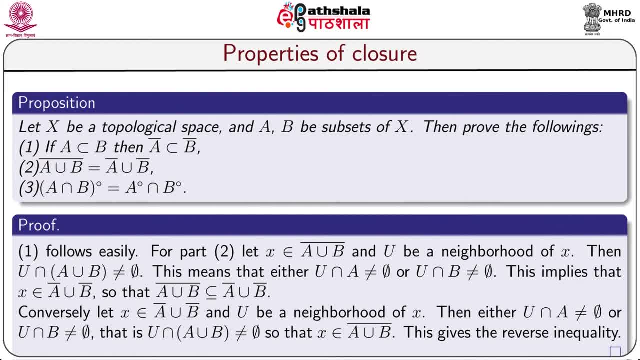 Number two: A union B bar will be equal to A bar union B bar. Number three: A intersection B interior will be equal to A interior intersection B interior. The proofs are easy, Still we are telling. this One is obvious for part two. 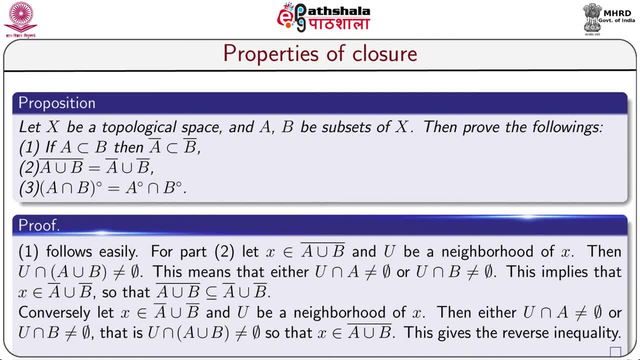 Let us consider x belongs to A union B- closure, and let u be an open set containing x, Then by definition, obviously u intersection A, union B is non-empty. This means that either u intersection A is non-empty or u intersection B is non-empty. 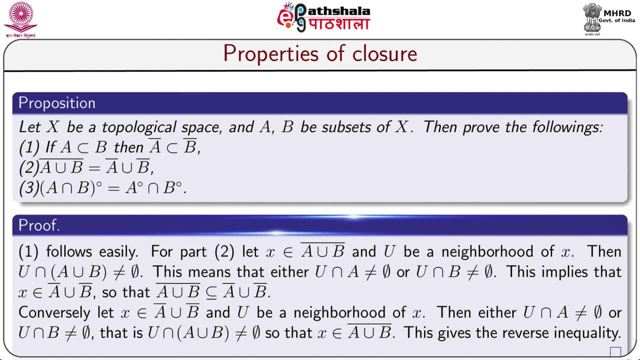 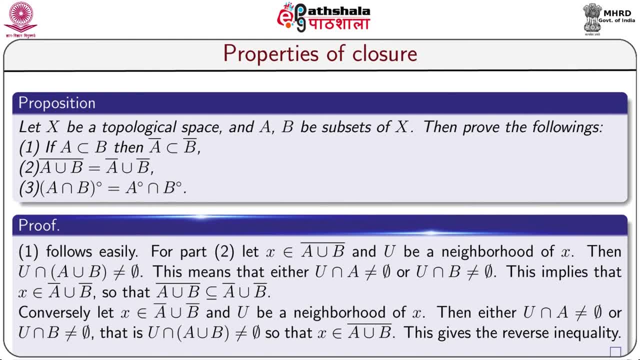 Conversely, let x belongs to closure of A union of B and u be an open set containing x, Then either u meets A or u meets A. Now, again from the front side, I have the result: x, bin requirements, and this is collector's. 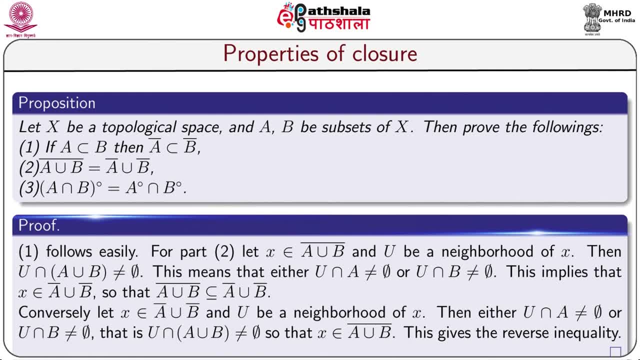 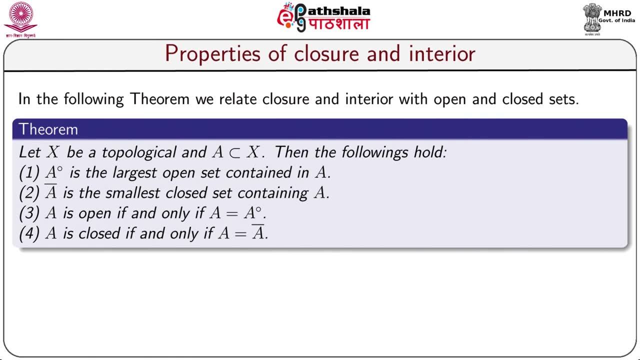 meets B, That is, you must meet union of AB. So X is a limit point of AB. So this gives the reverse inequality. The followings are some properties of closure and interior: Let X be a topological space and AB a subset of X. Then the followings hold: A interior is: 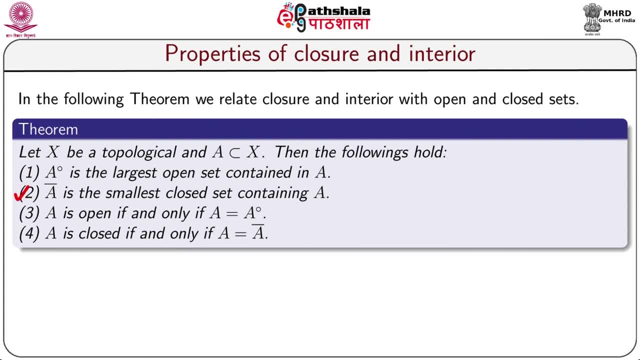 the largest open set contained in A. A closure is the smallest closed set containing A. A is an open set if, and only if, A is equal to A interior. A is a closed set if, and only if, A is equal to closure of A. So let us start the proof. 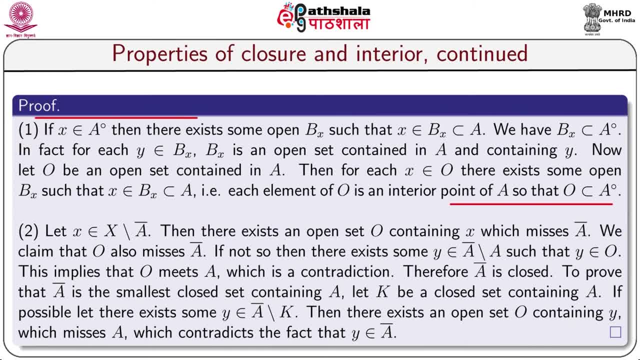 Number 1.. If X belongs to A interior, then there exist an open set B, such that X belongs to A. Is it B? Is it B? Better say it is a closed set. If A is a closed set, it is. 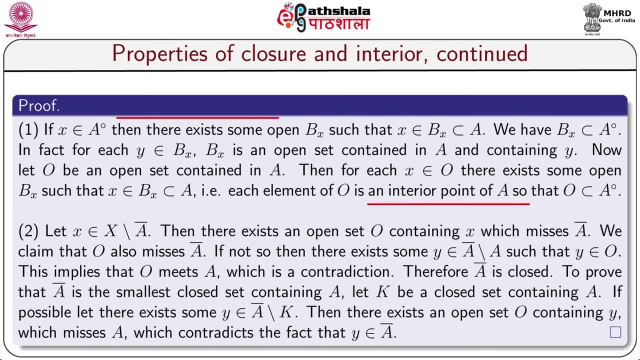 to be subset of A. We have that B is subset of A interior. In fact, for each Y belongs to B. B is an open set contained in A and containing Y. Now let O be an open set contained in A. Then for each X belongs to O, there exists some open set B such that X belongs. 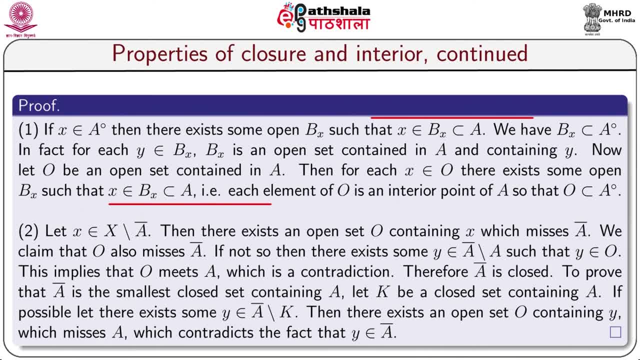 to B is contained in A. This follows from the definition, That is, each element of O is an interior point of A, so that O is a subset of A interior. The proof of the second Let X is in the complement of A closure. That means X is not a limit point of A. Then 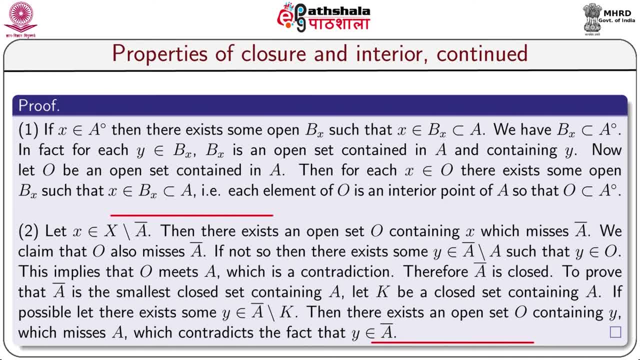 there exists some open set. So this is the condition for o containing X, which misses A closure, We claim that o also misses A. If not so, then there exists some Y belongs to A bar minus A, such that Y belongs to O. This implies that O meets A, which is a contradiction, Therefore A bar. 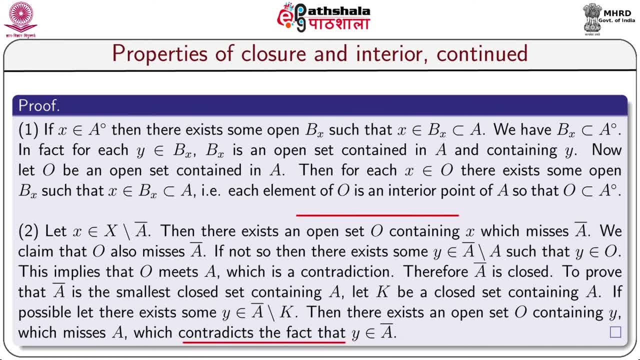 is closed. 2 b A bar is the smallest closed set containing A. Let K be a closed set containing A, If possible. let there exist some. Y belongs to closure of A minus K. Then there exists an open set, O containing Y, which misses A, which contradicts that fact that Y belongs to A. 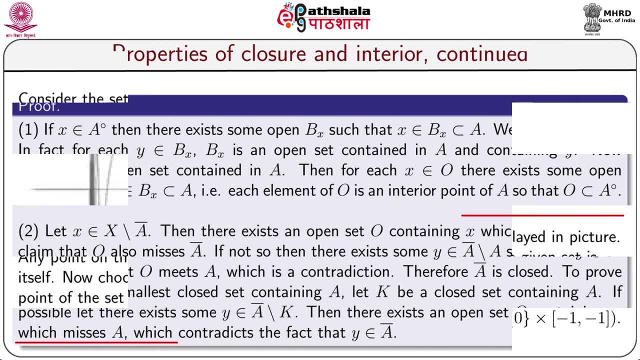 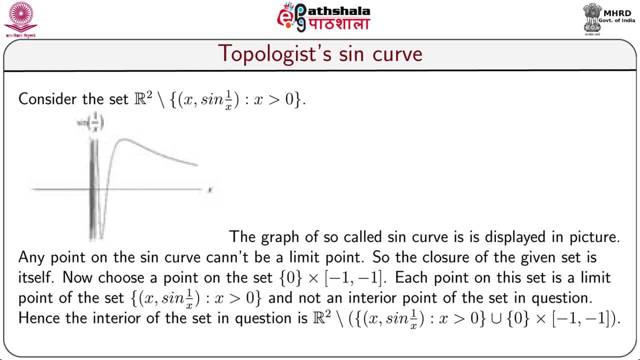 bar. This completes the proof of this theorem. This is an important, very important example. This is called topology sine curve. The graph is shown in the picture is called generally topology sine curve. Its description is that this is the all points x sine 1 by x, such that x greater than 0.. Now if this graph 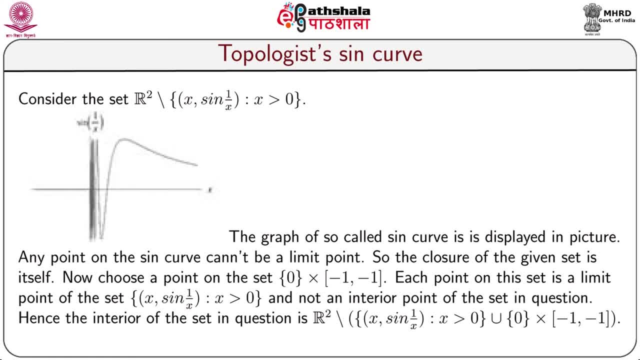 is removed from R2, what will be the interior enclosure? We can observe that if this graph is removed from R2, what will be the interior enclosure? If this graph is removed from R2, then its interior will be just this set, but its closure will include the set singleton. 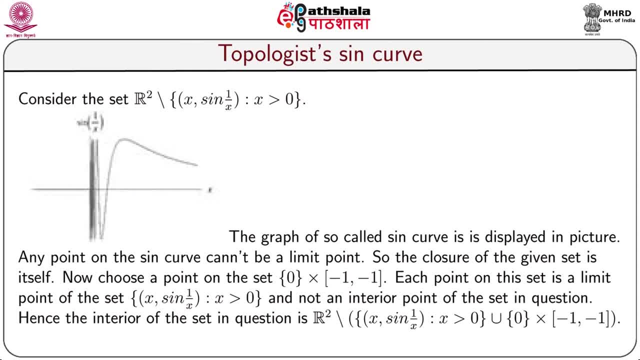 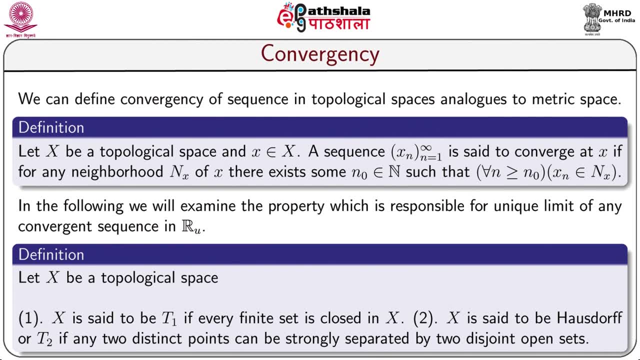 0 cross minus 1 to 1.. Now we will discuss convergency. Like elementary real analysis we can also define convergency here. We will define in this fashion a sequence: xn will be called converges converging to some point x. if for any open set containing x there exists some n0 belongs to n, such that 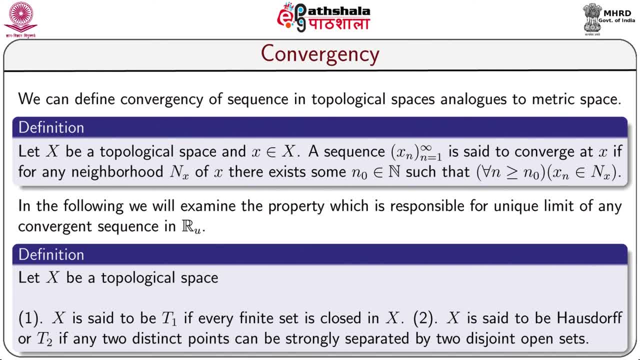 xn belongs to n for all n greater or equal to n0.. We have seen in the elementary real analysis that a sequence converges to only one limit point, if at all it converges. whether it also holds in arbitrary topological space or not, we will examine. 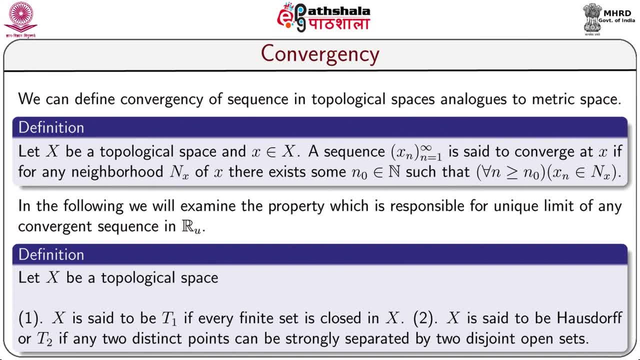 But before that we will define two notions of topological space or two properties of topological space. Definition: let x be a topological space, then x will be called T1. space is a. If every finite set in X is closed, number 2, X will be called house drop or T2 if any. 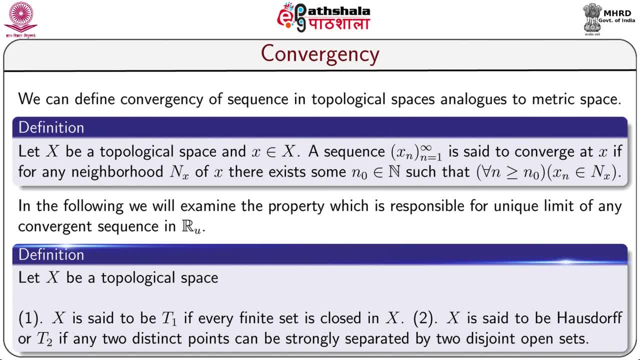 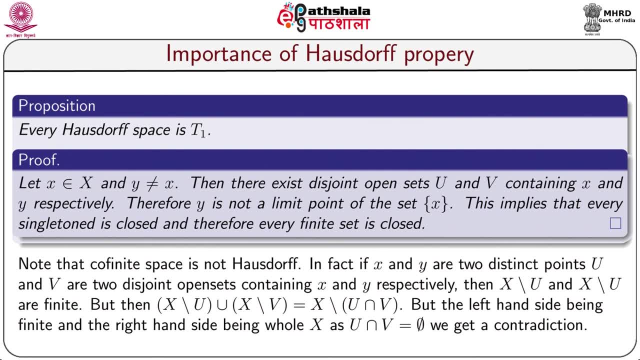 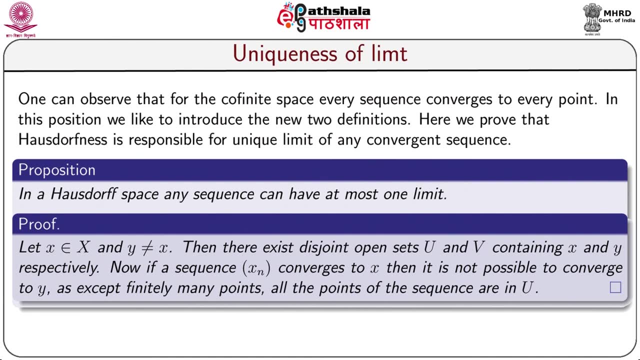 two distinct points can be strongly separated by disjoint open sets. This is very easy to show that every house drop space is T1. This is done in the slide. Now, if we observe that in co finite space any sequence converge to any limit point, 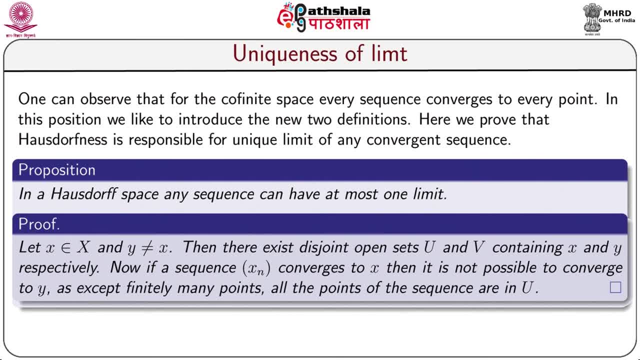 Why this happens? Because co finite set is not a house drop space, But in a house drop space a sequence can converge to at most one limit it. So we can get this following proposition: In a house draw space, each sequence can have: